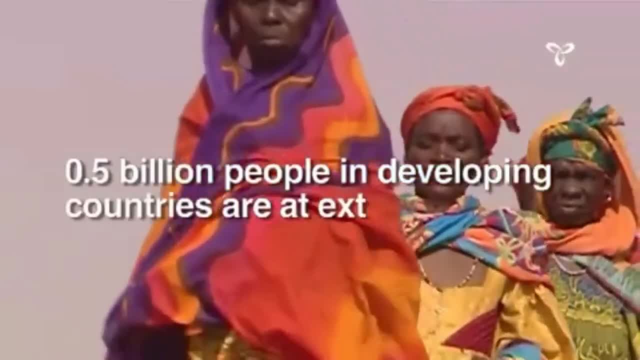 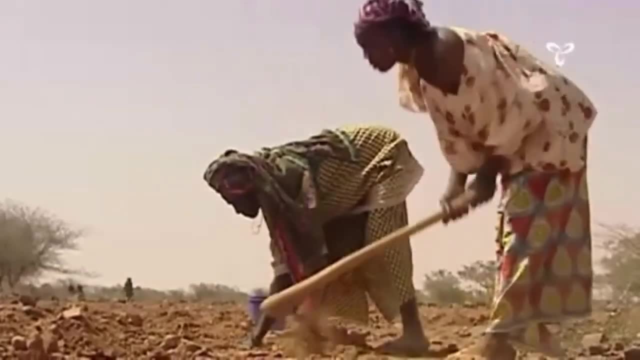 climate change. Half a billion people in developing countries are at extreme risk, many of them in some of the poorest areas of the world, such as sub-Saharan Africa, according to the 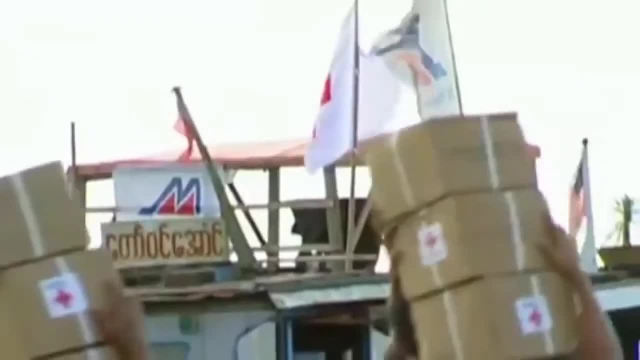 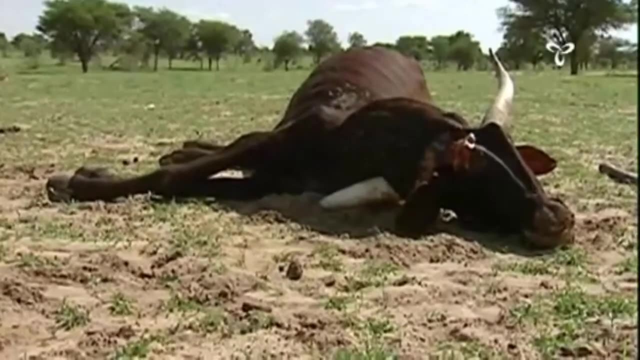 report's findings. Humanitarian aid provides relief in many emergencies, but it's not always the best answer to the problem. It's not always the best answer to the problem. It's not always the best answer to the deadly crises brought about over time by climate change, such as drought. 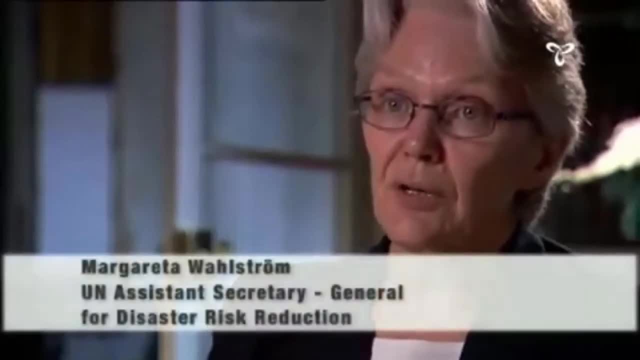 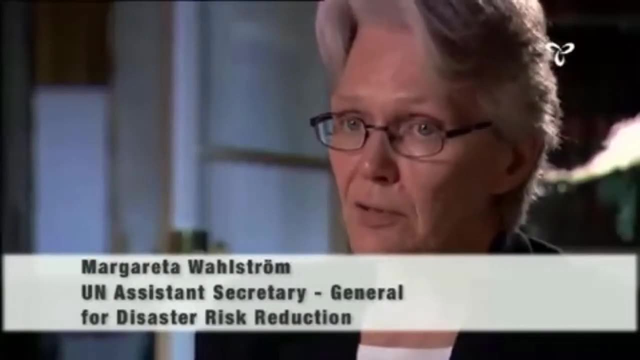 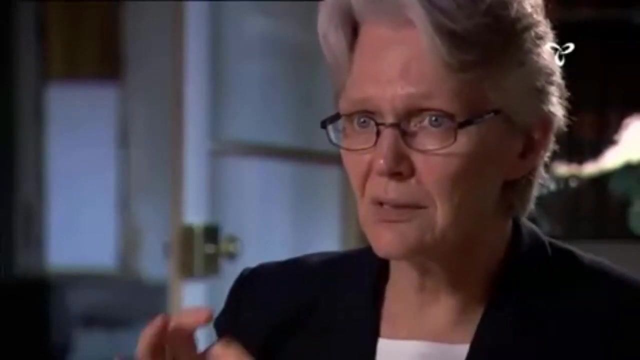 It's not always the best answer to the deadly crises brought about over time by climate change, such as drought. That's one of the disasters that we understand least about. And also the one that the international community has had great difficulties of coping with, and that's probably one reason why it is so deadly that it has been treated as a disaster, but it's a fundamental development issue. 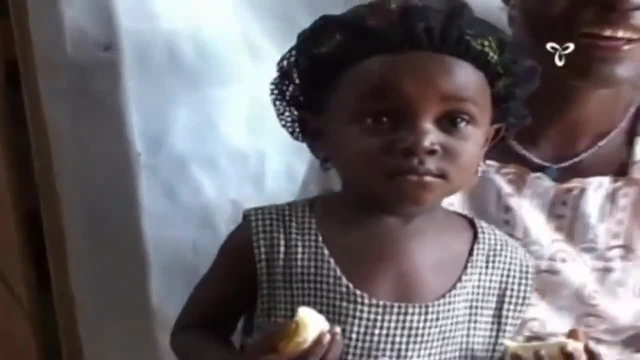 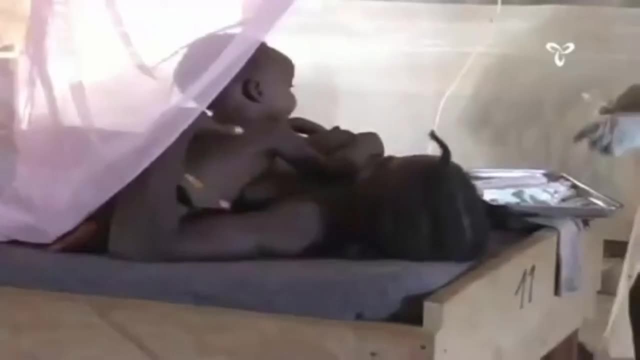 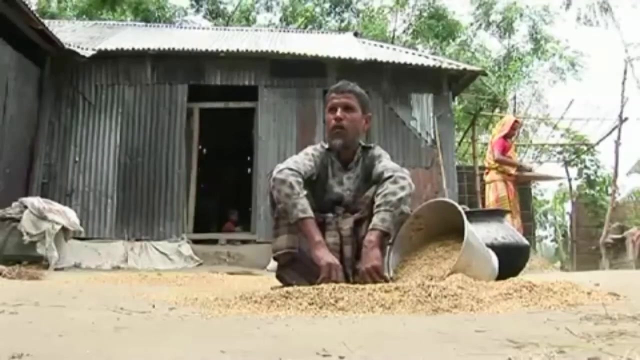 The report puts a human face on climate change by putting people on the streets. According people at its heart. Rather than underscoring abstract scientific data, it's the first comprehensive study specifically focused on the adverse effects of climate change on human society. It aims to be meaningful to the general public and useful to policymakers. 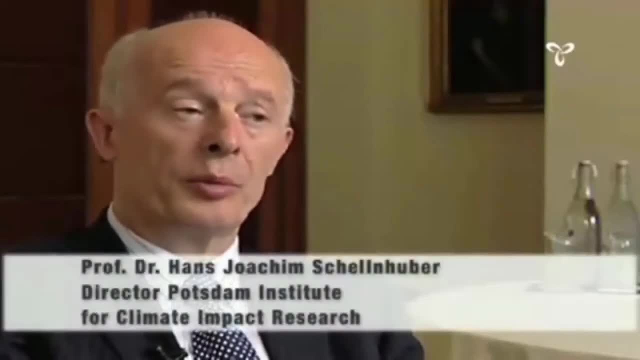 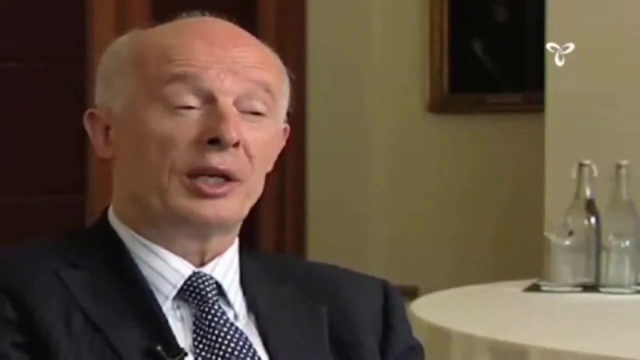 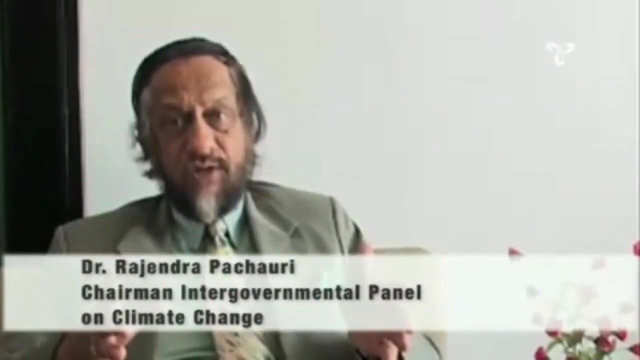 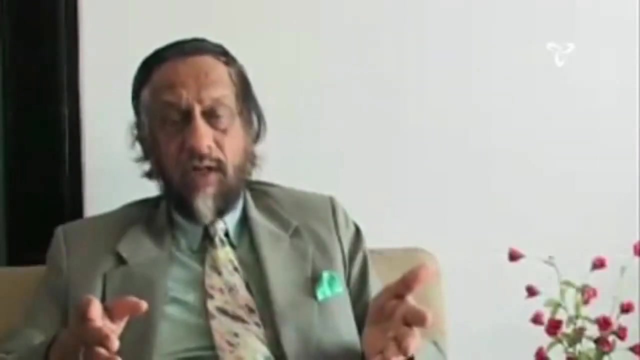 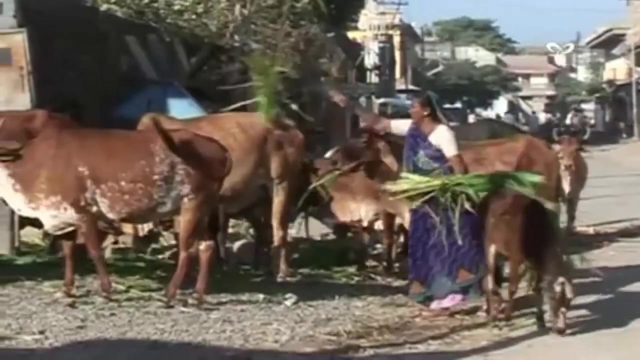 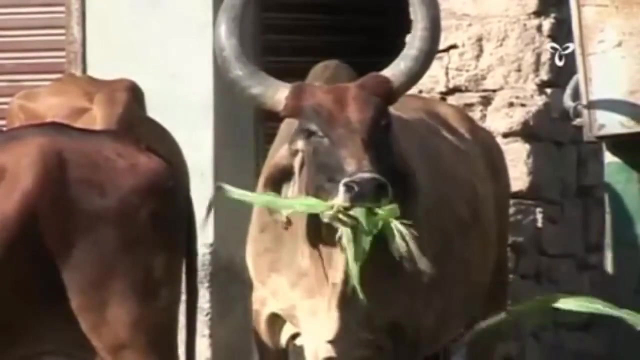 I mean, this report is a starting point, clearly. It will in particular prompt many people in the research community, but also among the organizations, to take it more seriously, the issue. And we have to get our acts together now. This is where we have to tell the world that unless we look at the humanitarian dimensions of the problem, then clearly we are likely to have a disruption in society in several parts of the world. We are even likely to have failed states. Developing countries bear more than 90 percent of the burden of climate change while contributing least to the causes, the report states. Ninety-nine percent of deaths linked to climate change occur in developing countries, which often emit the lowest carbon emissions. 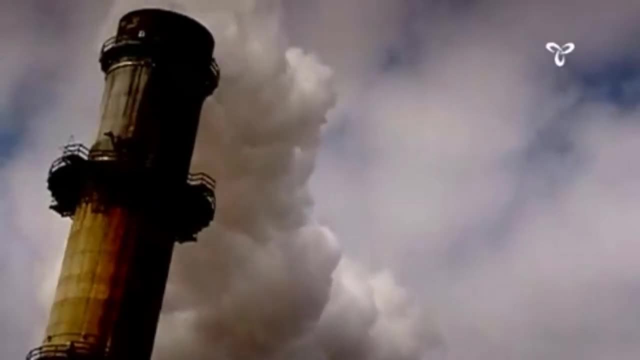 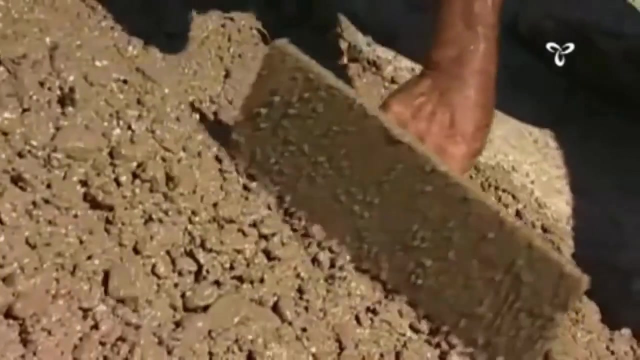 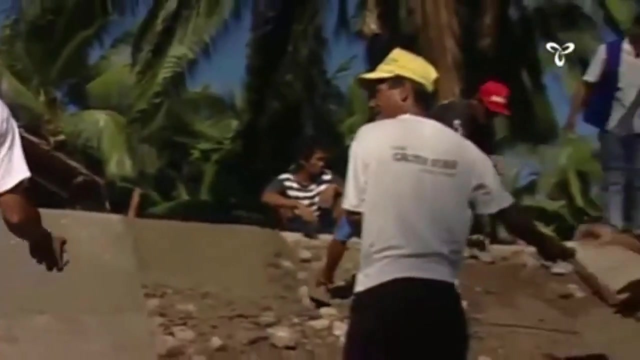 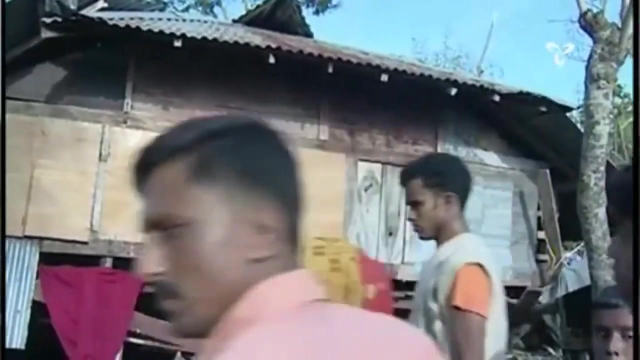 The report comes at a critical time, just six months before a new deal is due to be thrashed out by negotiators in Copenhagen to set new levels on emissions. Current adaptation efforts to reduce the human impact of climate change were woefully inadequate and needed to be scaled up a hundred times. Despite the dramatic consequences of climate change outlined in the report, it warns that its findings are very conservative and the true human impact is likely to be far more severe. 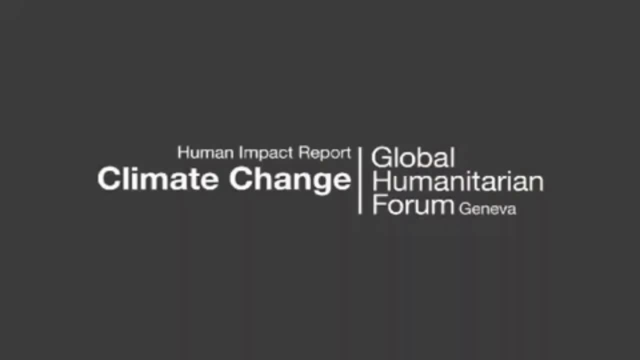 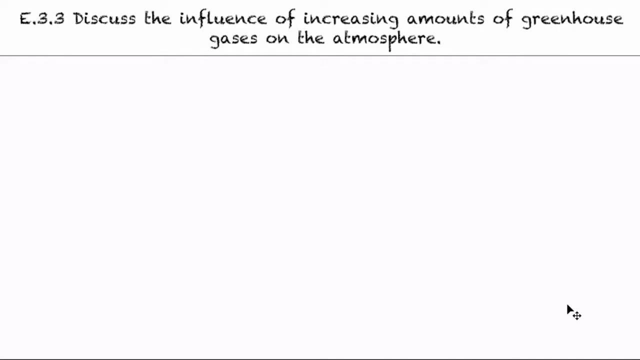 In today's topic, we are going to discuss the influence of the increasing amounts of greenhouse gases on the atmosphere, and in other words, just what are the effects of climate change. And in there you can see that actually we are already experiencing some of these changes. It's just that a lot of us in the developed world are not actually having to experience them first hand. And there's actually another documentary called The Age of Stupid, which although it's not a great documentary, what it does do well is it takes different news clips that have happened over the last decade or so, and pieces them together in such a way that you see all these sort of seemingly 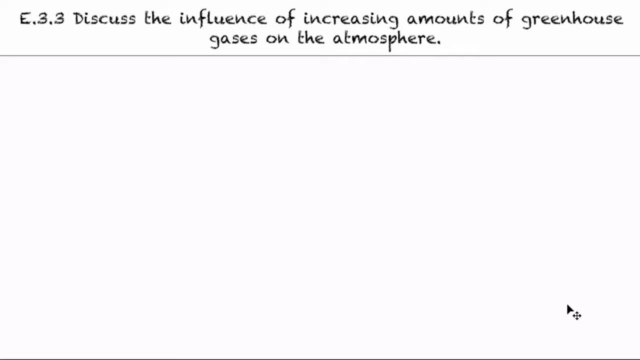 independent events. But you bring them together and then you get a clearer picture that the whole thing is going on. 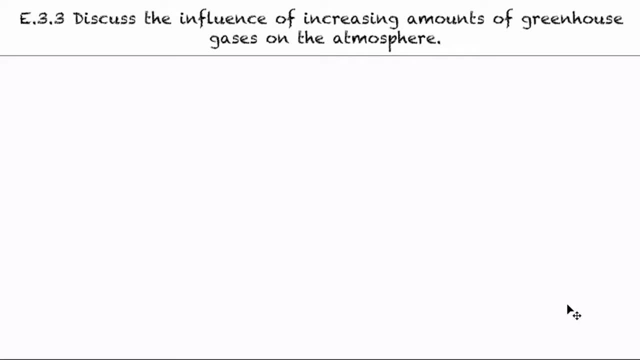 And the question it begs is, will people look back to us and say this was sort of the age of stupid, because all this knowledge we have, why aren't we making changes? And a lot of that can come down to many, many reasons, including the way our brains have evolved 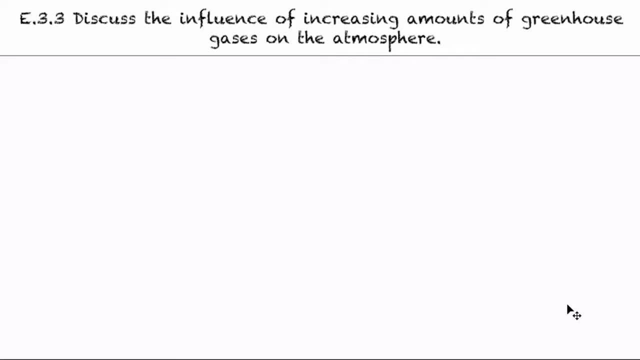 to not be able to comprehend long-term change or value long-time consequences, as opposed 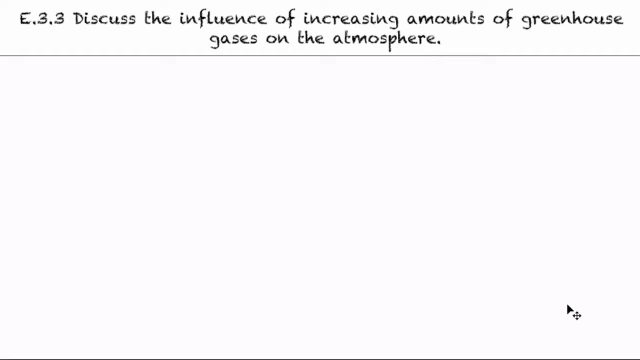 to short-term gain. But let's just take a look at what the UIB is looking for when you're discussing the influence of the greenhouse gases. So the first thing they're looking for is to talk about the thermal expansion of the 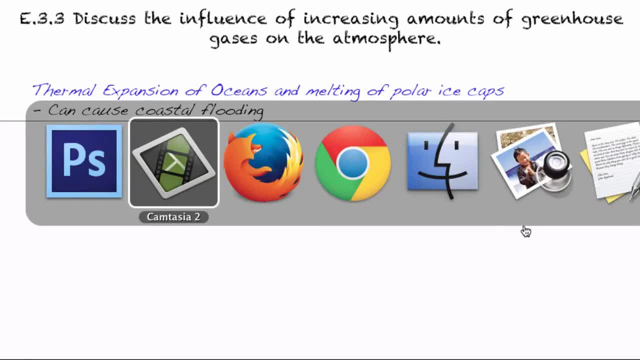 oceans. Now what that basically means is that as particles get warmer, they spread apart. 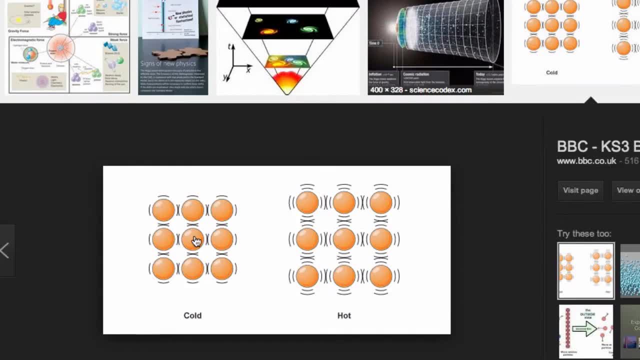 So let me just illustrate that with a simple model here. So colder water, as it warms up, the space in between will... 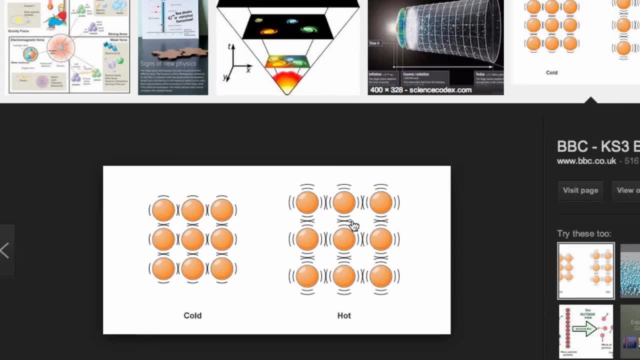 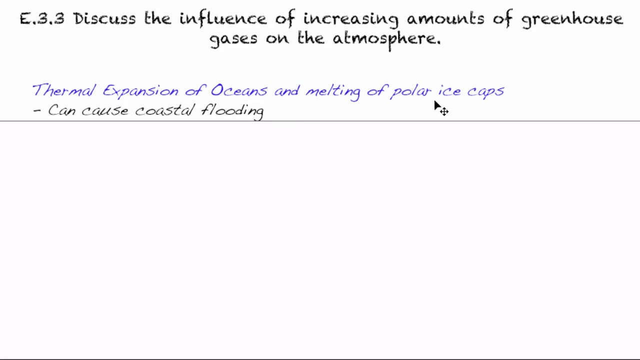 expand. So if you imagine the size of the ocean and how many particles of water there are, that adds up to a lot of volume. So that would cause the sea level to rise. Another reason for the sea level rise, it would be the melting of the polar ice caps. And what happens in that case is water that is now locked above surface, like as ice, it's not adding to the volume of the ocean. Once it melts, then it's going to add to the volume of the ocean, because it will be part of it. So both of those can cause the coastal flooding. 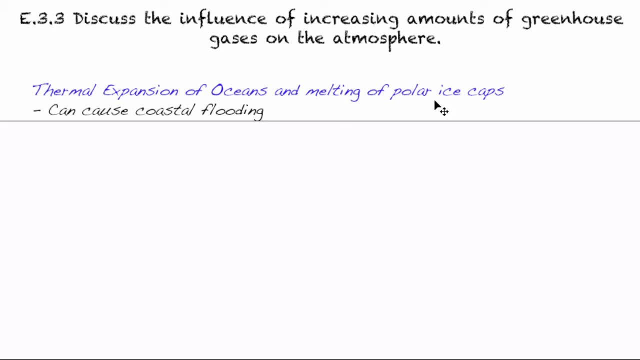 And as a quick aside, there's also a few pieces related to this. As the oceans warm, whereas temperature of any fluid rises, its solubility of gases decreases. So in other words, right now, as the ocean's temperature is increasing, it's actually going to be able to hold less carbon dioxide. 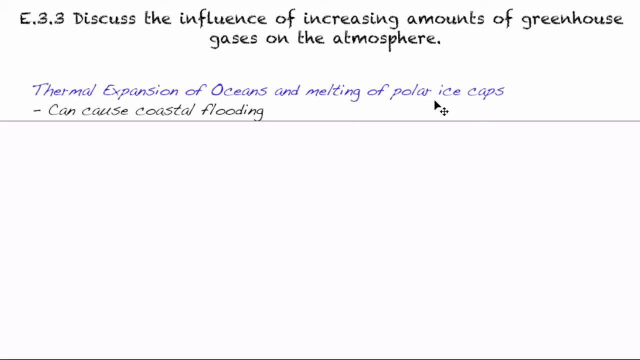 So as the ocean's temperature rises, it will release more carbon dioxide, which will drive more climate change, which will drive more release of CO2, etc., etc. In terms of the polar ice caps, because they're white, they reflect a lot of light away from Earth. If they melt, then there will be more absorption of the light instead of reflection, and that can actually, again, cause more re-radiation of infrared, which can be absorbed and re-emitted by the greenhouse gases. So those are what we call polar ice caps. Subtitles by the Amara.org community 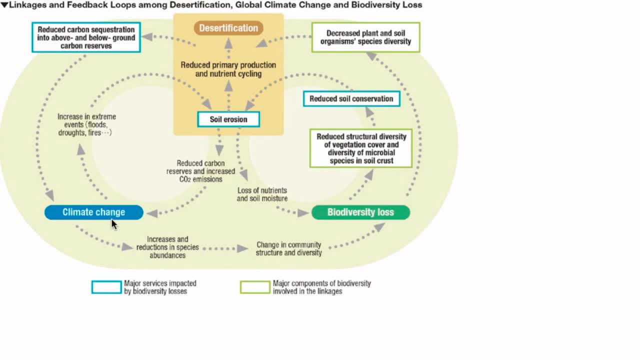 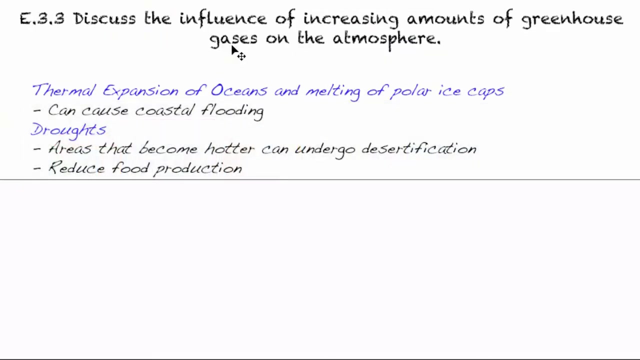 Ah, we'll go in more in the soil topic, but climate change can affect biodiversity, and if there's a decrease in biodiversity, that can impact the soil, and that can drive erosion into certification. At the same time, climate change with floods and droughts can also drive erosion into certification. cm So with that, we get to reduced food production. Subtitles by the Amara.org community Loss of Food Productions merchandise 1 became a significant chord 오빠 with the project some years ago, and the development last year. For over a year of quantification, the project created a new study project titled etwa esto noке Proskerrumbius, and it was left